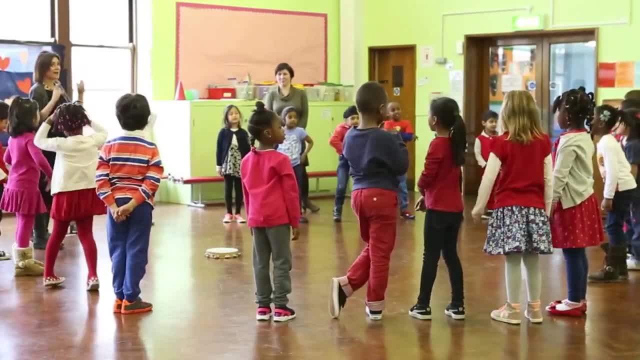 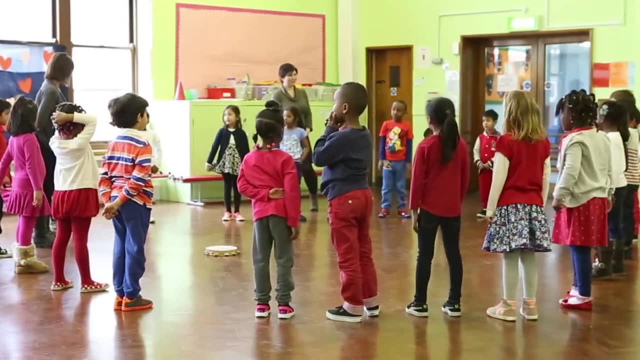 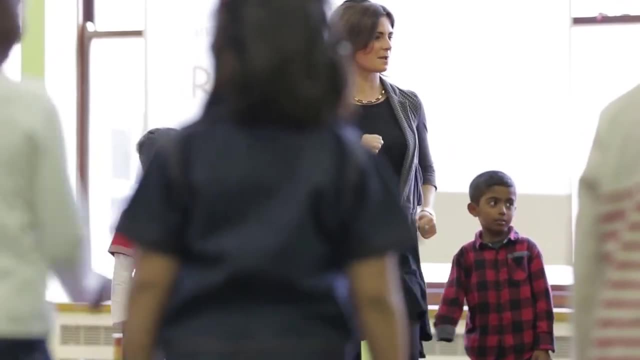 Good morning everybody. Good morning Missy, Good morning everyone. H-E-L-L-O. H-E-L-L-O. This is how we say hello. This is how we say hello. Move your feet to the beat. Move your feet to the beat. 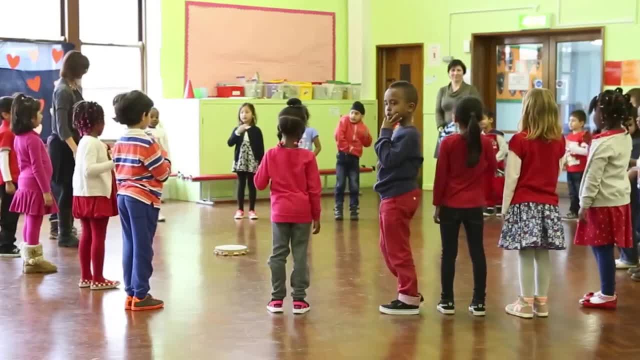 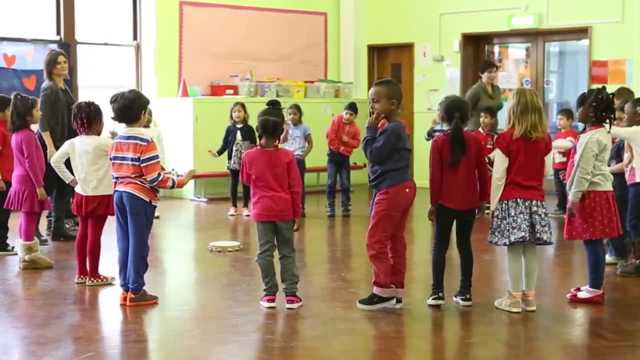 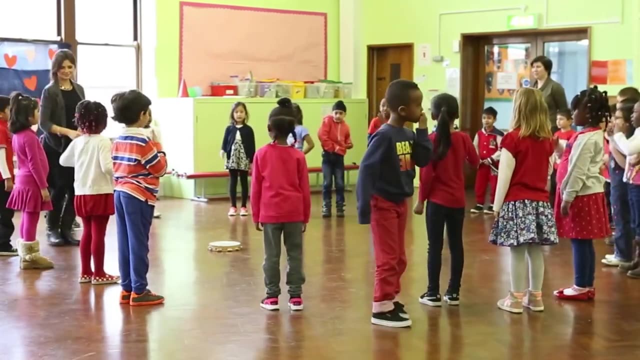 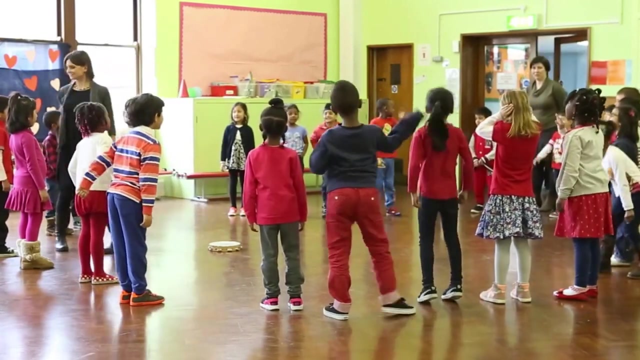 Can you feel my heartbeat? Can you feel my heartbeat? H-E-L-L-O. This is how we say hello. This is how we say hello. Move your feet to the beat. Move your feet to the beat. Can you feel my heartbeat? H-E-L-L-O. H-E-L-L-O. This is how we say hello. This is how we say hello. 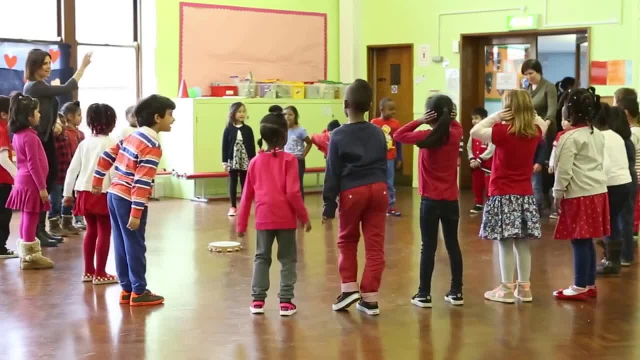 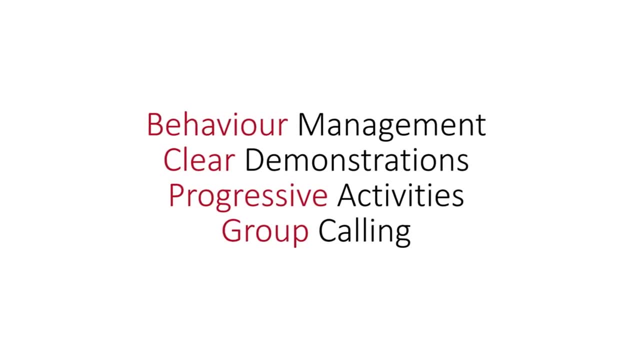 Move your feet to the beat. Move your feet to the beat. Can you feel my heartbeat? H-E-L-L-O, H-E-L-L-O. This is how we say hello. This is how we say hello. This is how we say hello. 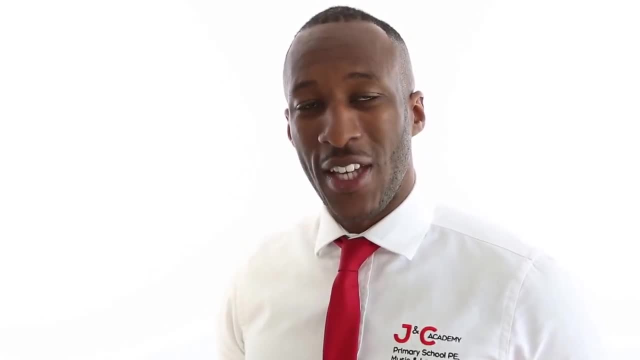 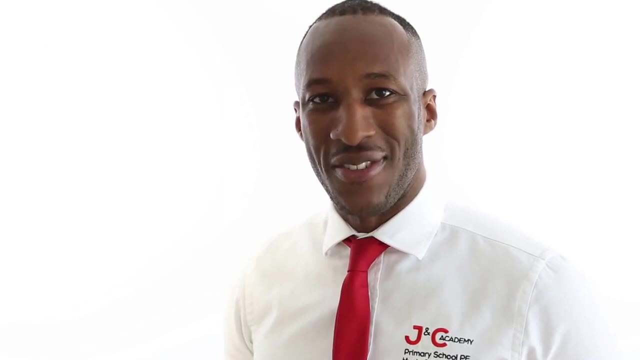 In the main phase of the lesson, the teacher reinforces the expectations for behaviour before providing a clear demonstration which helps children to improve their performance. Notice how Molly delivers activities which are dynamic and progressive and which clearly link to the main learning objective. She often uses the group calling technique so that all children can learn together. 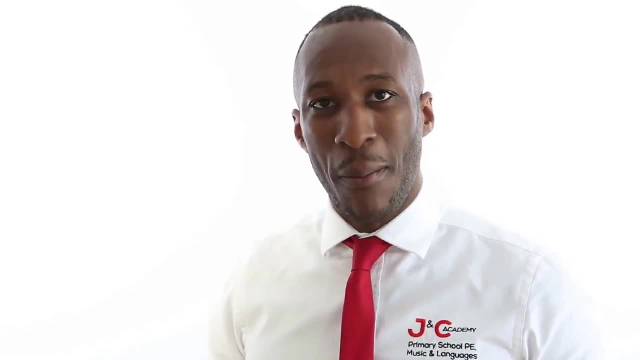 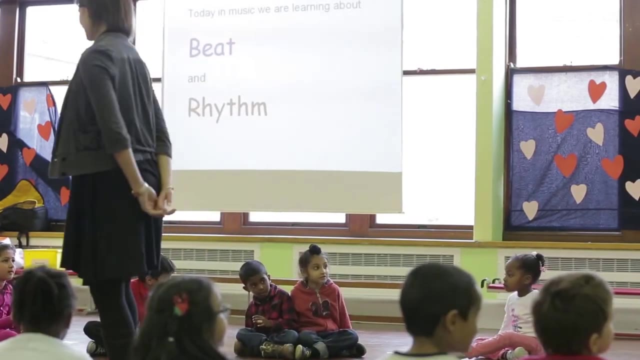 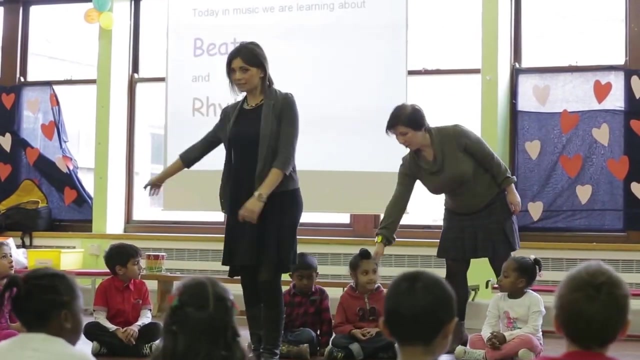 She also uses the group calling technique so that all children can learn together and help them remember key words. Show me good sitting everybody And no talking. So we all know this song. When the music stops, you need to quickly run to the middle of the circle and you need to play the beats. 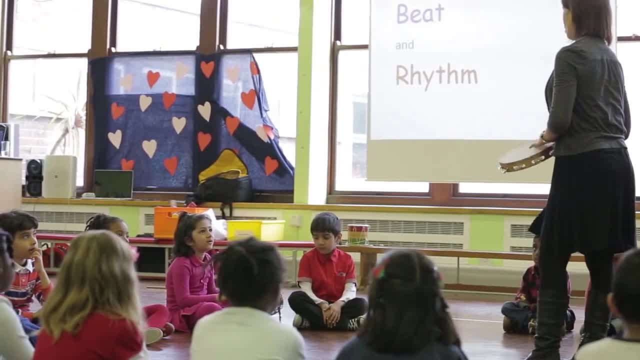 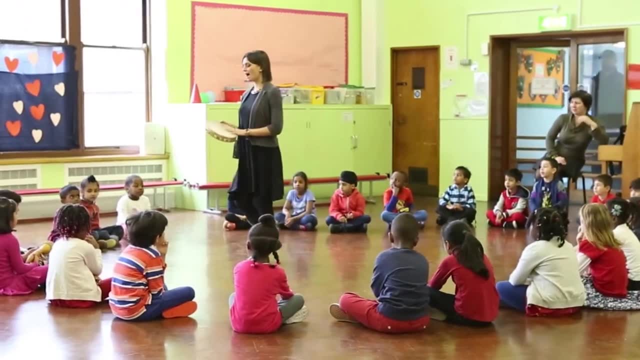 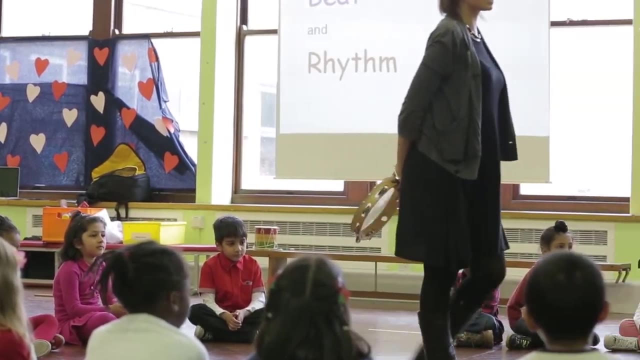 The beats or the or the rhythm: rhythm. okay. so if we're going, I can play the tambourine. tambourine, was I tapping the beat or the rhythm? somebody tell me, yeah, I was doing the beat. if I was to do this, you can play the. 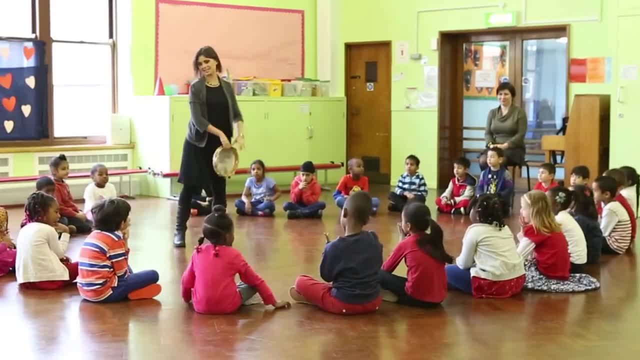 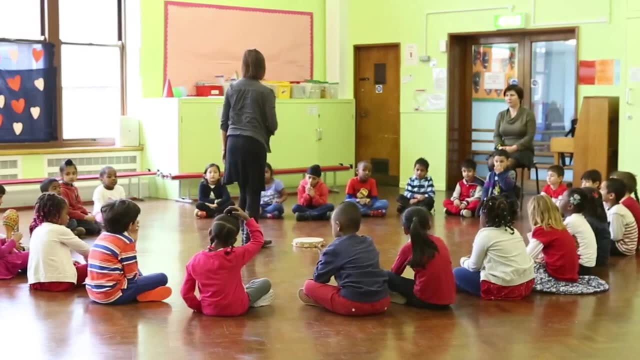 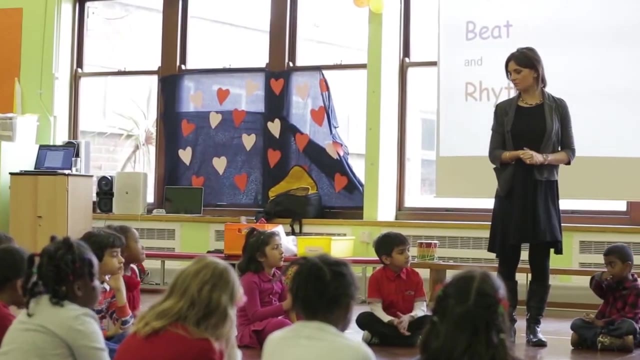 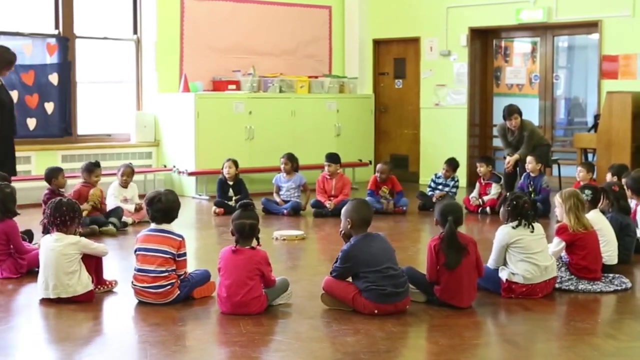 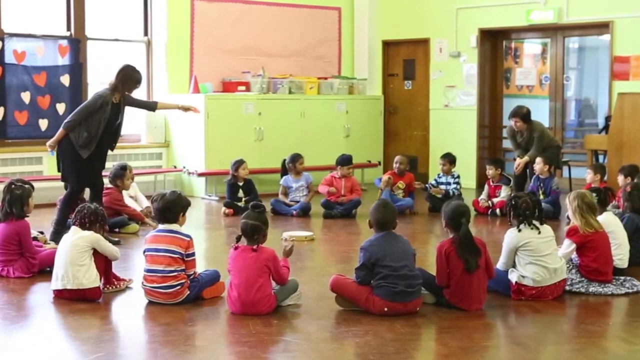 tambourine. that is rhythm. fantastic. so if the music stops, you are going to do either the beat or the rhythm. now I'm going to tell you which one to do. okay, so I want to see if you can do the difference between beat and rhythm. it didn't stop. press it on. it didn't stop, did it quickly. 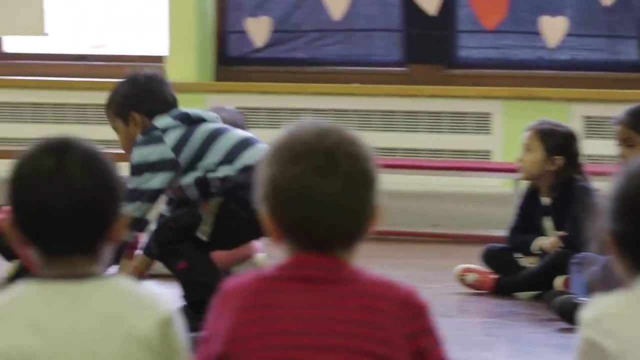 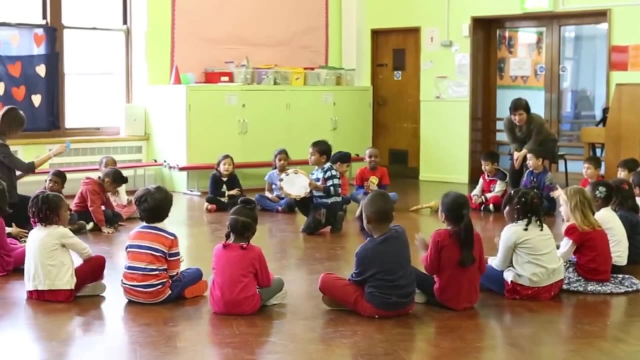 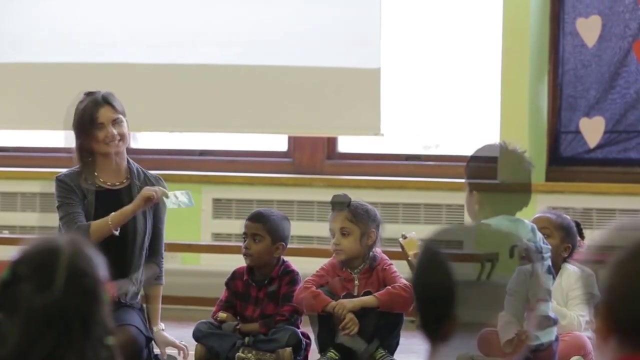 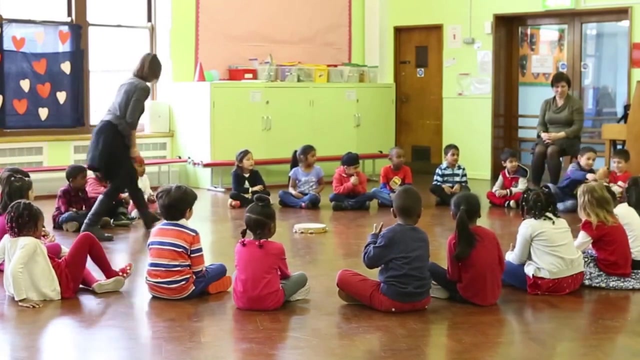 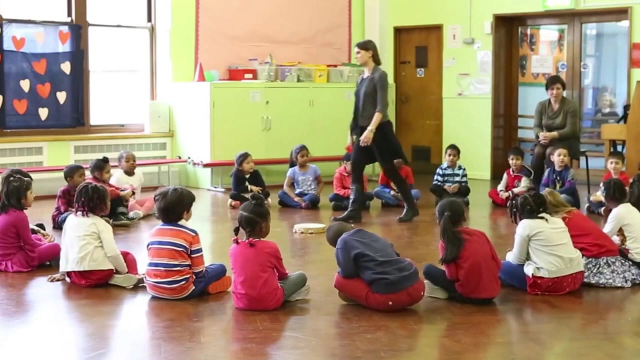 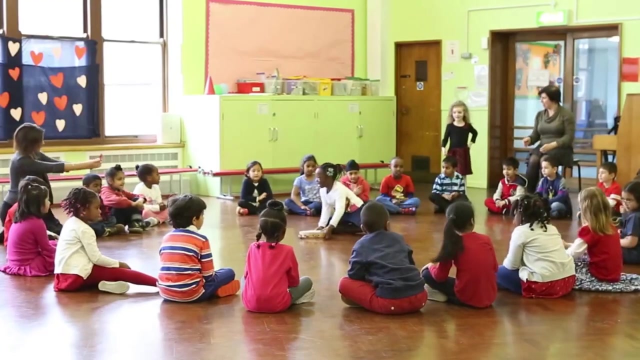 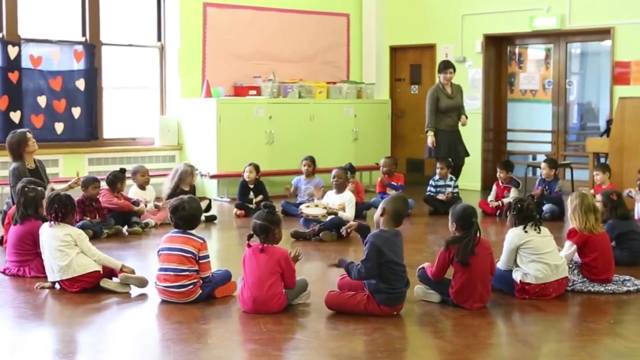 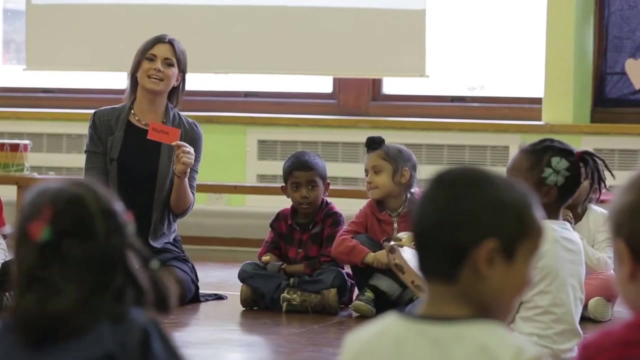 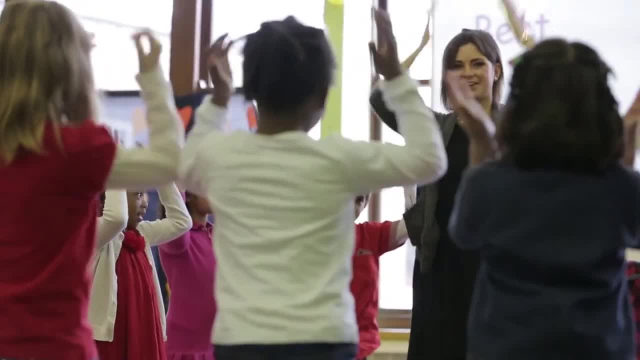 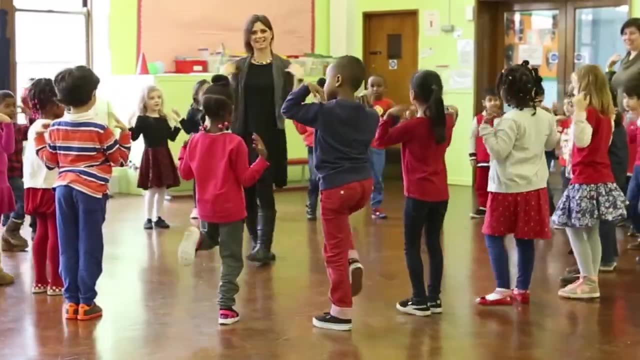 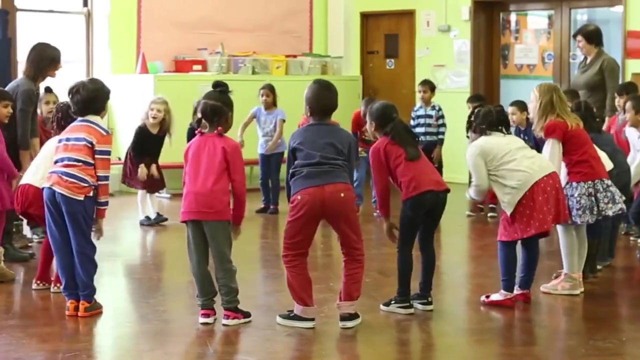 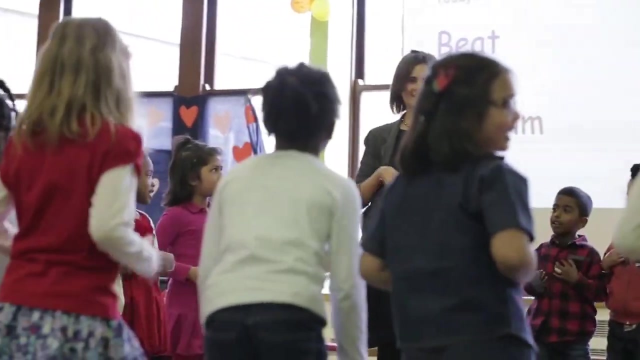 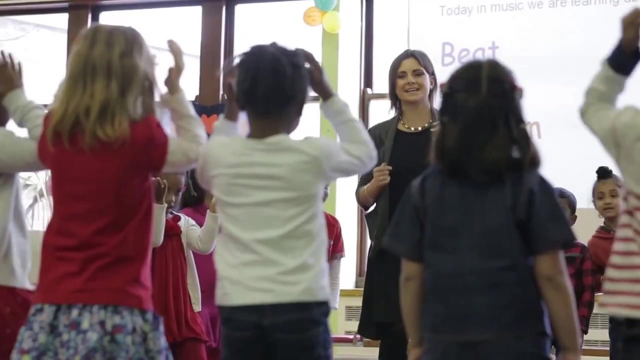 well done, sing che che cule. che che cule. che che Che Che Covinta, Che Che nichts 長ato arnya. somebody tell me. what are we tapping in time to? we're tapping to the beat. well done. now we're gonna do it again, and I really want you to sing even louder this time ready. 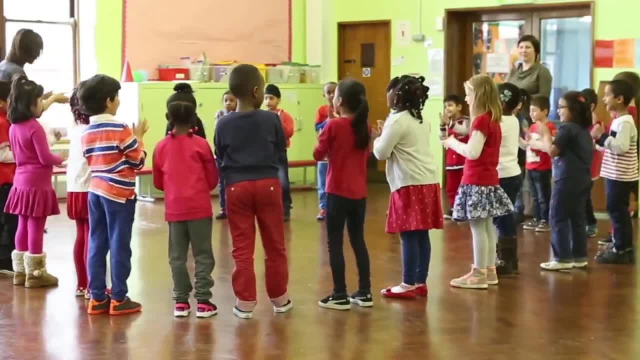 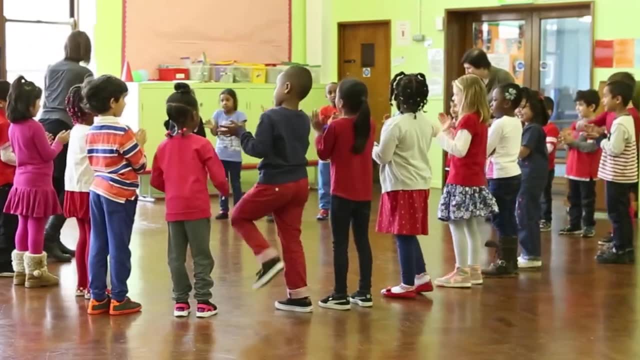 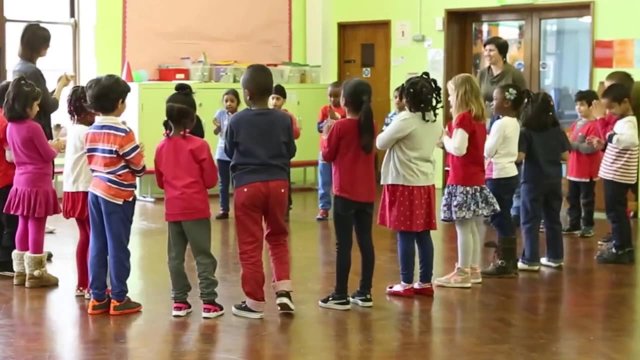 Che Che Cooley, Che Che Cooley, Che Che Covinsa, Che Che Covinsa, Covinsa, Langa, Covinsa, Langa, Caca, Chilanga, Caca, Chilanga, Com Adende, Com Adende, Com Adende, Hey, 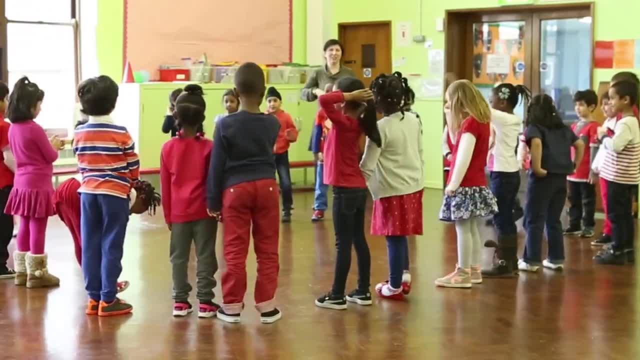 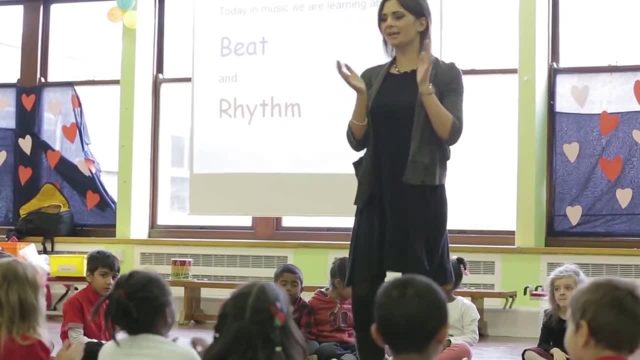 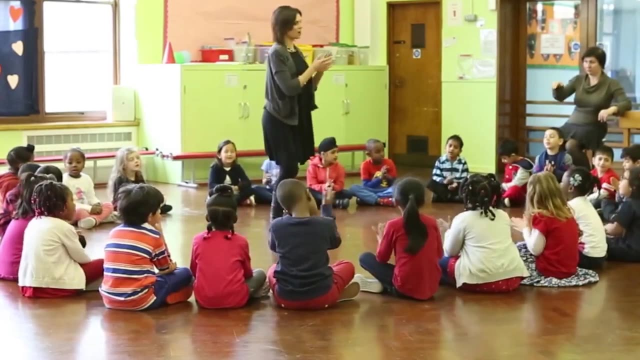 Fantastic and freeze This old man. he played one. he played knick-knack on my drum with a knick-knack paddywhack, give a dog a bone. this old man came rolling home. Beat or rhythm, don't shout out. 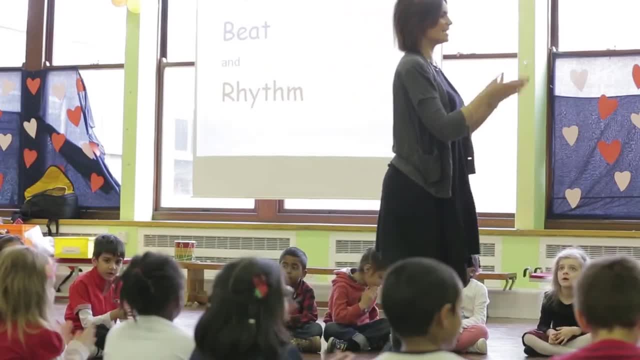 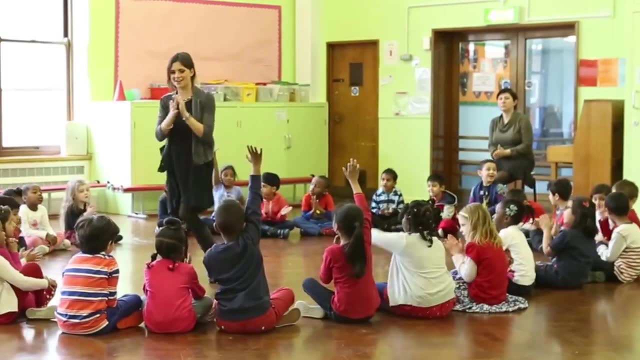 Beat. well done This old man. he played one. he played knick-knack on my drum with a knick-knack paddywhack, give a dog a bone. this old man came rolling home Rhythm. 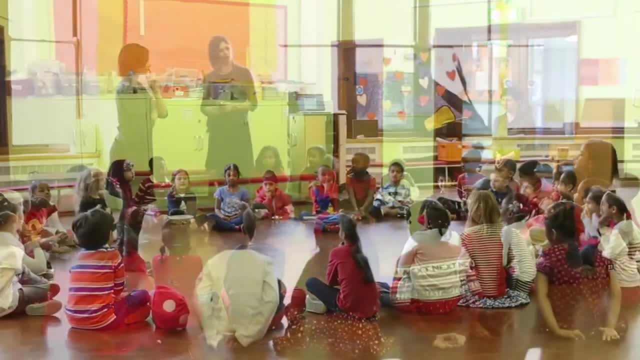 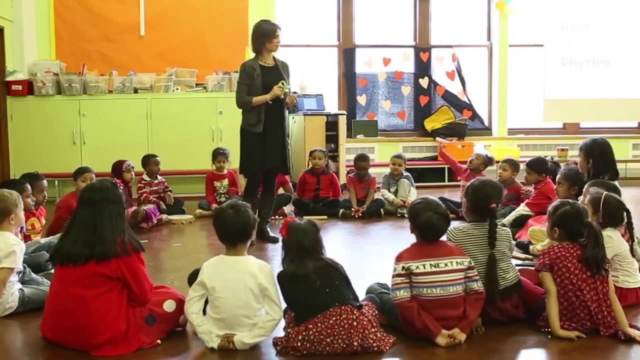 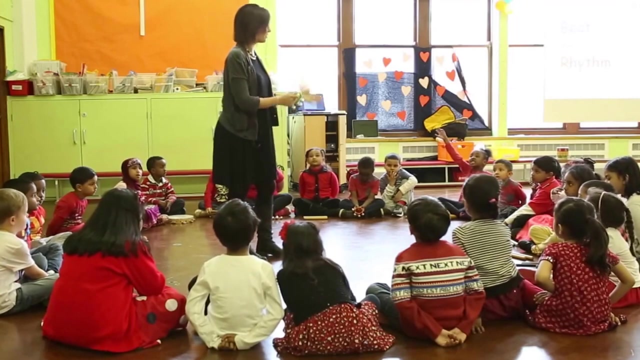 Rhythm. Okay, now show me, you go sitting. Can somebody tell me if I am playing the beat or the rhythm? Listen, Okie-tokie on da, okie-tokie on da rhythm. And then we're going to go. hexacolour, missile warning, it's what is it? 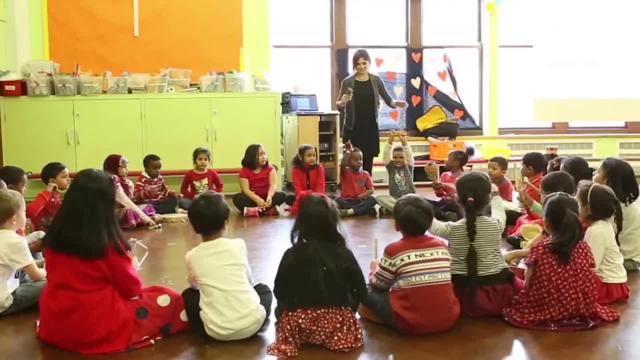 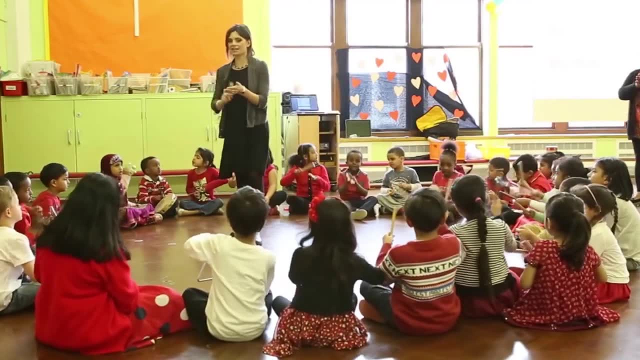 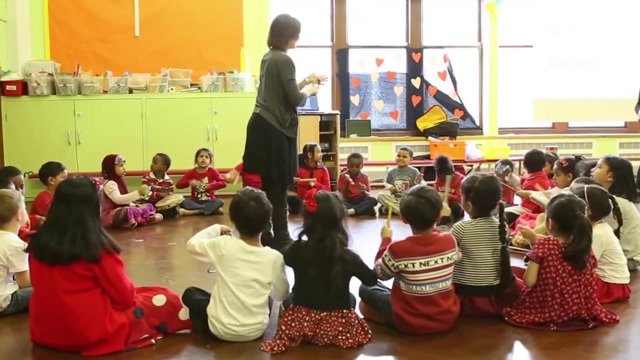 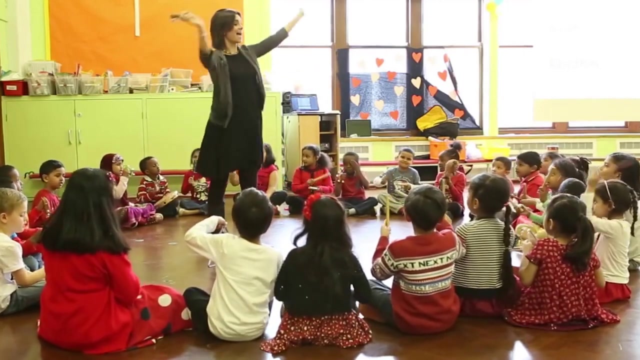 Speed Speed. Get ready, Speed Speed. Can I just squeeze through So rhythm ready? Okie-tokie on da okie-tokie on da Hey, mister J, mister J. Rhythm. Okie-tokie on da okie-tokie on da hey, mister J, mister J. 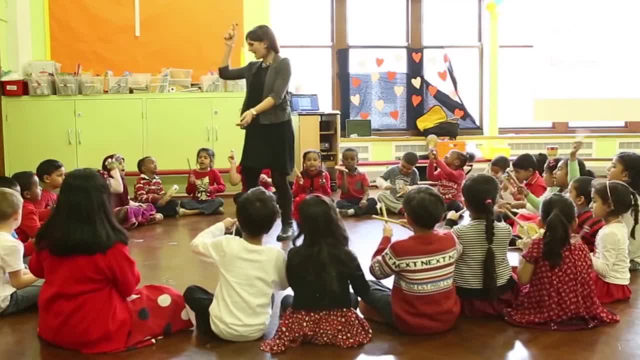 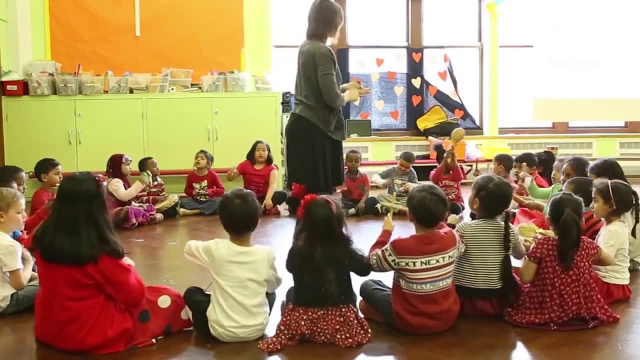 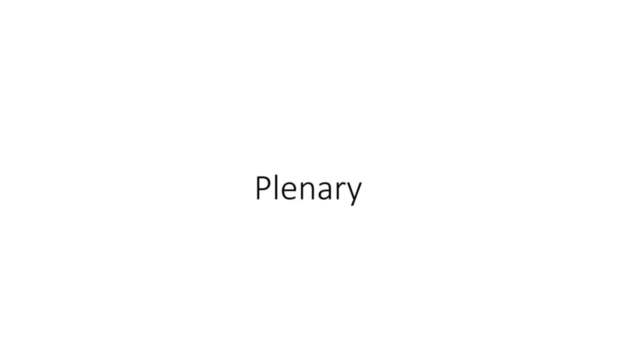 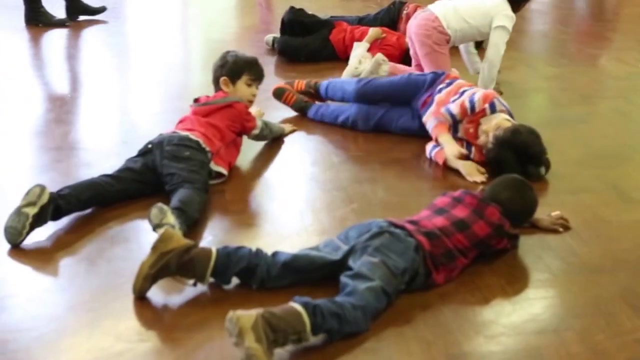 Beat Hexacolour missile warning. Beat Hexacolour missile warning. Well done, I'll keep talking on that. I'll keep talking on that. hey, Mr Bear, Mr Bear, Mr Bear. At the end of each lesson, the teacher asks pupils to close their eyes and reflect on. 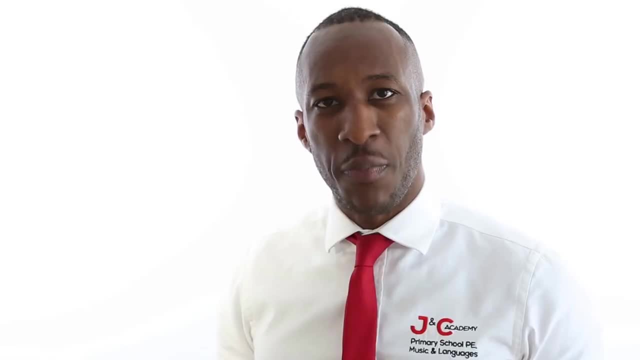 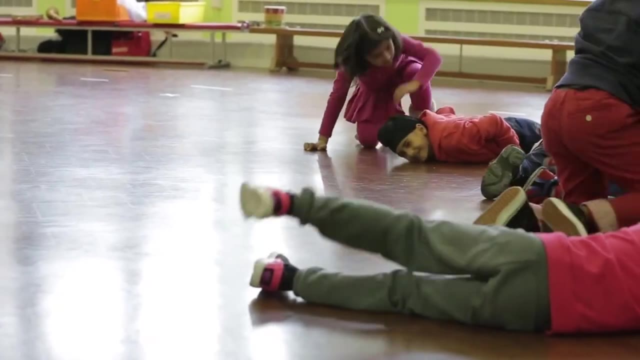 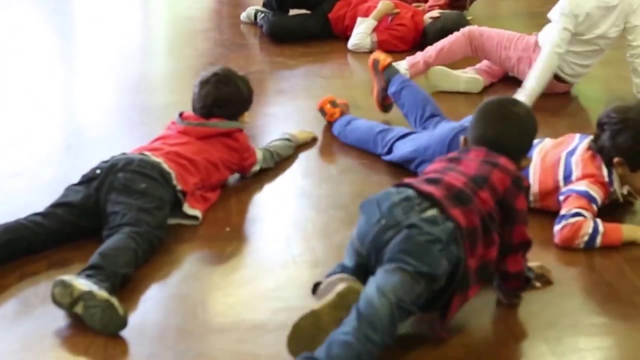 what they learnt, helping to ensure that all pupils are calm and inspired before their next lesson. Now slowly start to wake up everybody slowly. Shhh, Come on really slow, Really slow. Good, Good, Good, Good Good. 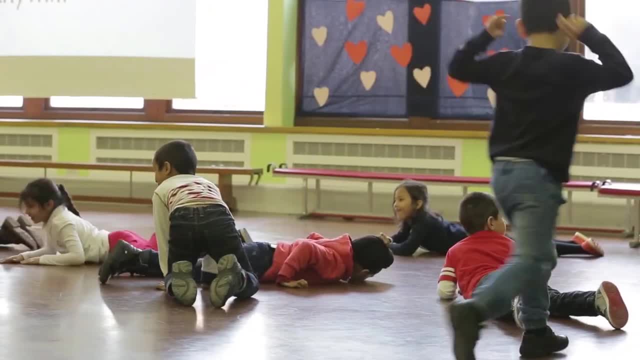 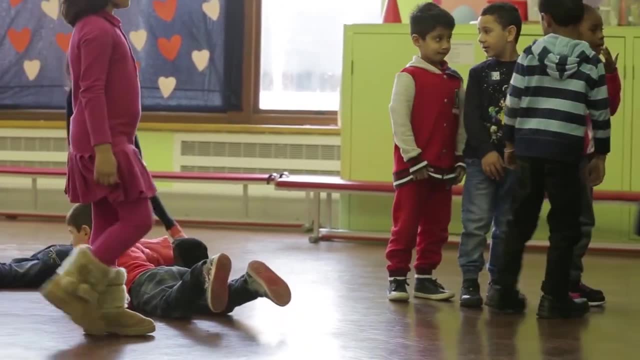 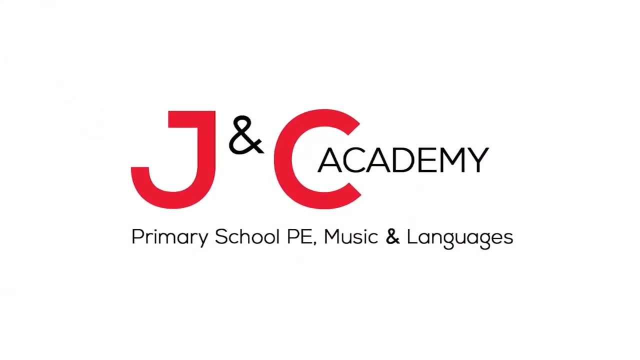